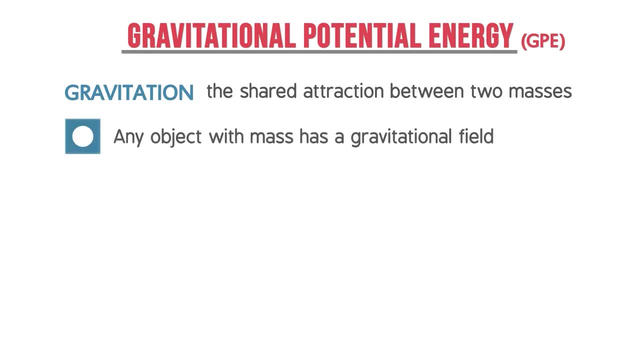 In fact, gravitational potential energy is the energy that is produced by the particle. In fact, any object with mass has a gravitational field which acts on and influences other bodies of mass. Hence GPE is created by the gravitational field. In everyday life, one of the most prevalent gravitational fields is produced by the Earth. 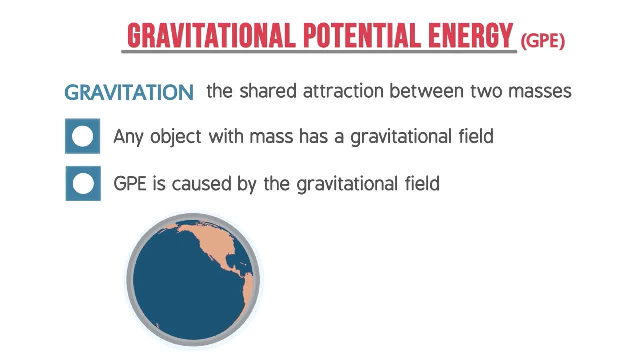 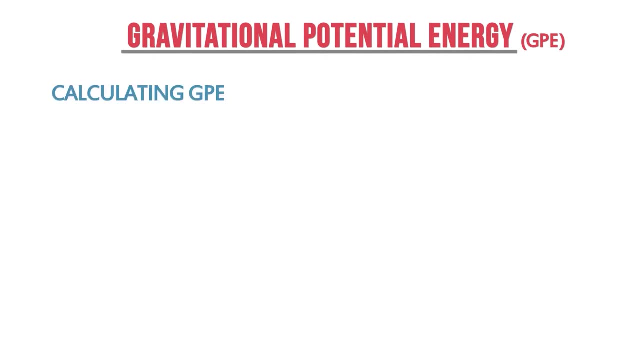 And we know that Earth's gravity field generates a force with an acceleration of approximately 9.8 meters per second squared. This gravity field also causes objects that are moved away from the Earth's surface to gain gravitational potential energy. We can calculate the magnitude of an object's current gravitational potential energy by: 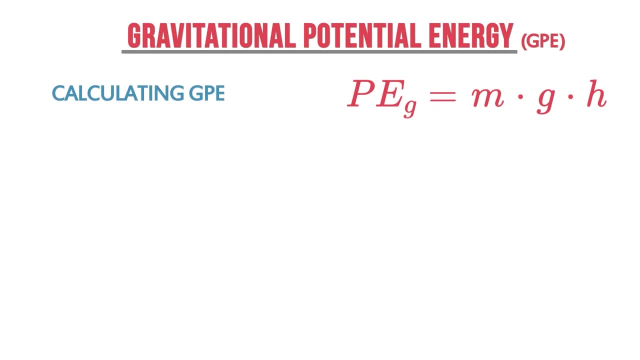 using the formula, PE equals M times G times H. And let's explore this formula in detail so we can shed some light on the concept of gravitational potential energy. First is M, which stands for the mass of a single object or a system of objects. 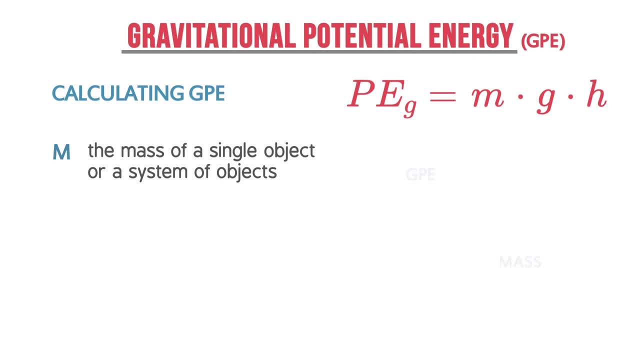 The mass M affects the potential energy. So let's take a look at an example. We have a system of objects in which we have a mass of a single object. The mass M affects the potential energy- energy of the object positively. This means that the higher an object's mass, 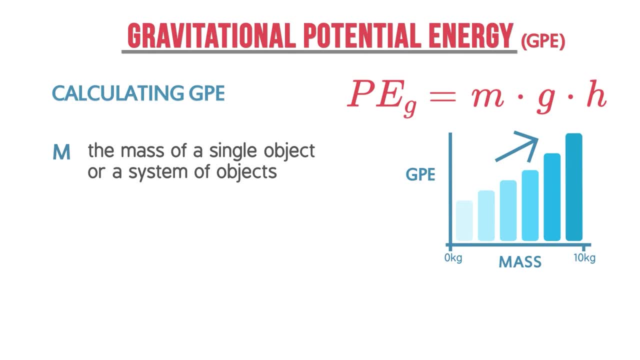 the more gravitational potential it will have. Next, the G stands for the acceleration of gravity, which is negative 9.8 meters per second squared, And note that gravity has a negative coefficient because it is going in the downward direction. Finally, H stands for the height away from the surface or the 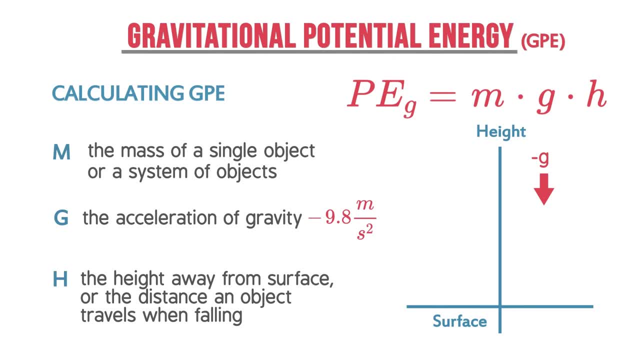 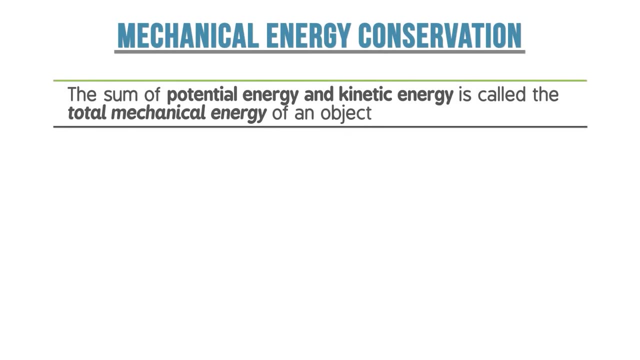 distance an object travels when falling. In this case, the higher values for the change in height results in greater potential energy. This is why the energy that an object has is by virtue of its position relative to the surface of the earth. The sum of potential energy and kinetic energy is called the total. 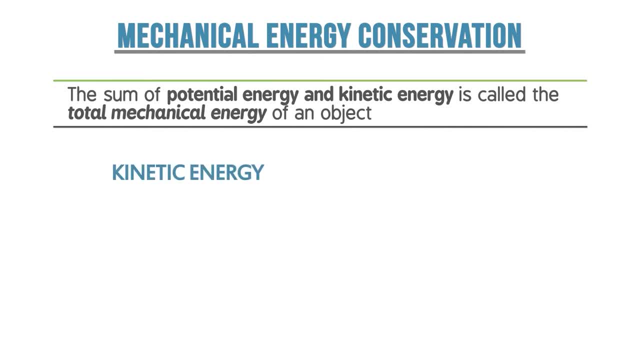 mechanical energy of an object, where the kinetic energy is energy that is possessed when an object is in motion. The formula for kinetic energy is one half of the object's mass times, velocity squared. As mentioned earlier. energy changes from one form to another form of energy and energy changes from one form. 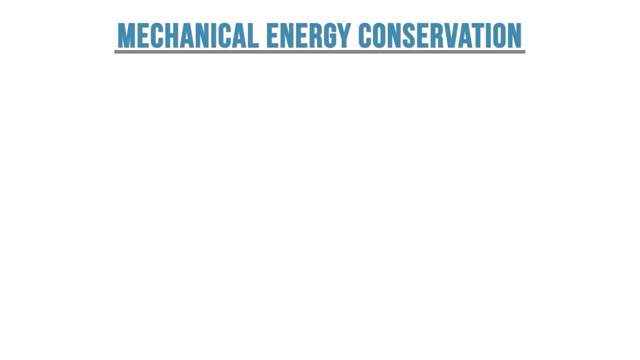 to another form of energy. It is never created or destroyed. Here's an example of how the conservation law applies to mechanical energy. When you take a look at a pendulum, you can assume that there is some kinetic energy in the pendulum simply because it is moving, Yet at the top of the swing the pendulum stops.